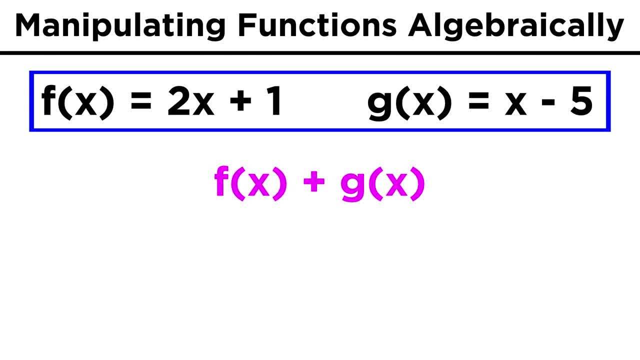 We could do f plus g of x, that's the same as f of x plus g of x, which is two x plus one plus x minus five. Combining like terms, we get three x minus four. We could do f minus g of x, which is f of x minus g of x, or two x plus one minus the. 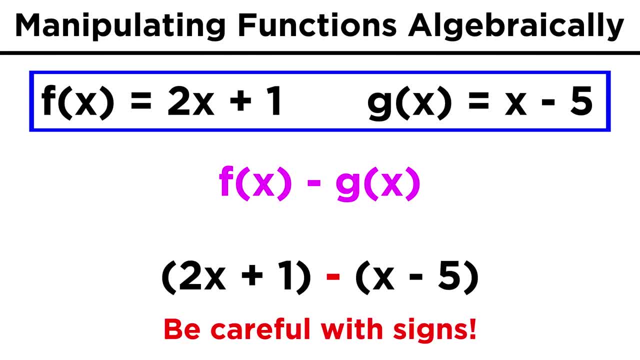 quantity x minus five. Don't forget to distribute this minus sign, which inverts the signs of these terms, giving us two x plus one minus x plus five, which becomes x plus six. If we did g minus f, we would get a totally different answer. 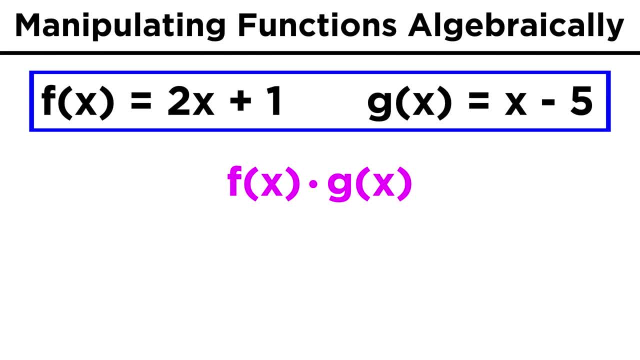 We can also do f times g of x, which is f of x times g of x. That would give us the product of two binomials which we could FOIL. We've already covered this method in detail, so hopefully we can do this quite easily to. 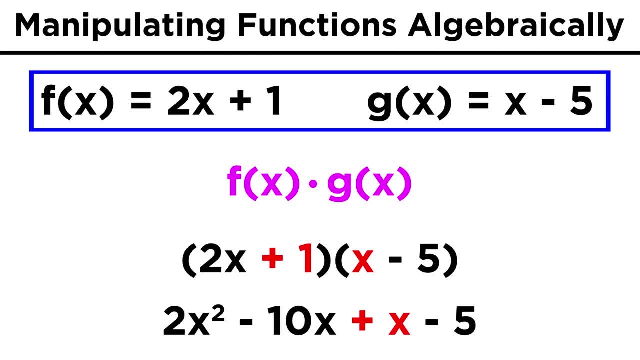 get two x squared minus ten, x plus x minus five, which we can then simplify by combining the x terms. And lastly, we can do f over g of x, which is f of x over g of x. In this case, we just put two x plus one over x minus five, and that's all we can do. 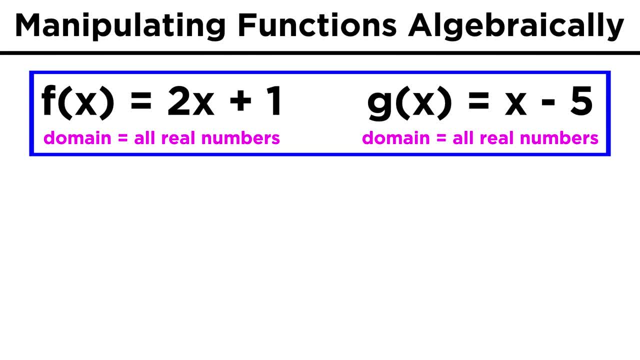 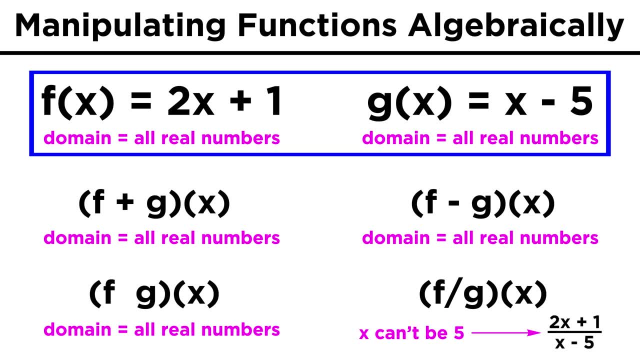 We should note that the domains of both f of x and g of x are all real numbers and that domain does not change for any of the above manipulations, except for the division we just did, Because with x minus five in the denominator, x can no longer be equal to five. 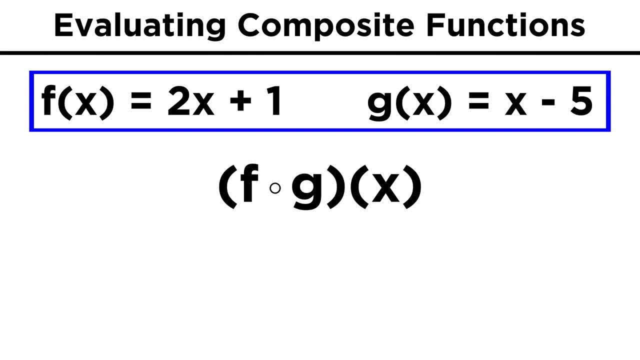 We could also evaluate composite functions. This is when we do something like f of g of x. Note this: with a little open circle or a little more logically, we can put g of x where x goes in: f of x. This is different than f times g, because we are plugging g into the function f.